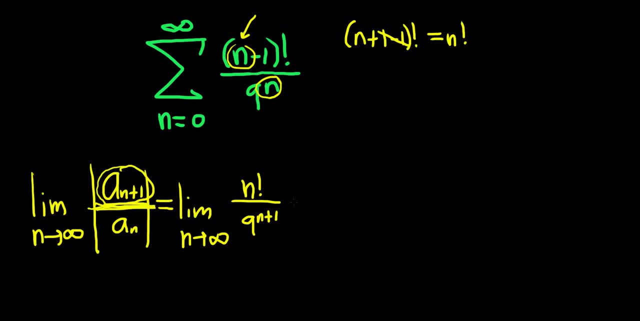 same thing as multiplication by the reciprocal. So typically what we do with the ratio test is put a time symbol here and then we just flip this whole thing, because that's the same thing as division. So this is 9 to the n over, and then we have on the bottom n minus 1 factorial. 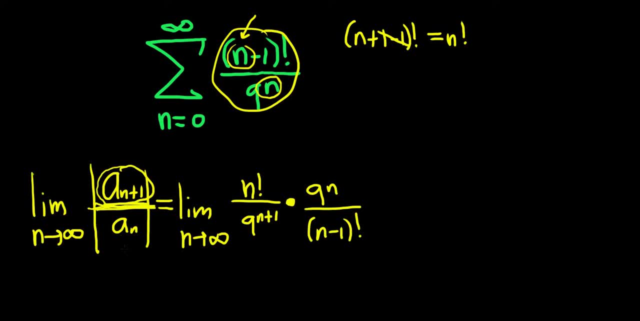 So again, first you plug in n plus 1, and then, instead of dividing by a sub n, we typically just multiply by the reciprocal. There's some simplification that goes on here, and let me just do it on the side up here. So first we have n factorial over n minus 1 factorial. 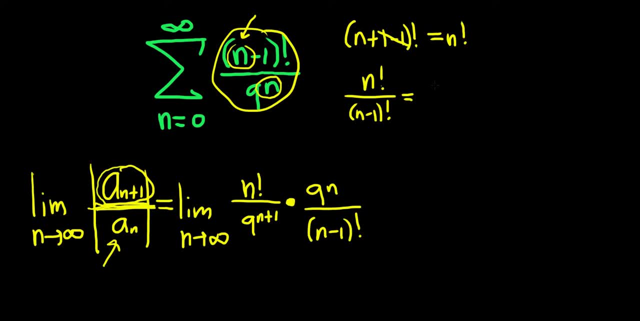 So n factorial is really n? n minus 1, n minus 2, dot dot dot 3,, 2, 1.. Then n minus 1 factorial is just n minus 1, n minus 2, times dot dot dot 3,, 2, 1.. So you see, all of this goes. 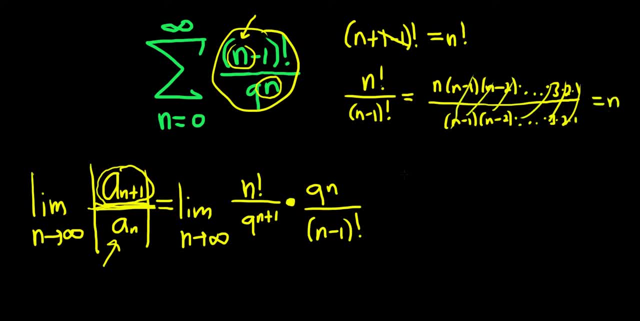 away. So you're just left with n. So this is equal to the limit, As n goes to infinity of n. And then what's up with the nines? So we have 9 to the n over, 9 to the n plus 1.. We could think of that as 9 to the n over. and here's the key. 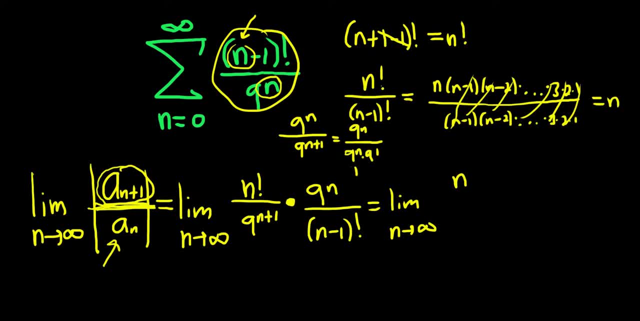 9 to the n times 9 to the 1.. Because when you multiply these you actually add the exponents 9 to the n times 9 to the 1 is 9 to the n plus 1.. It's because the bases are the same. 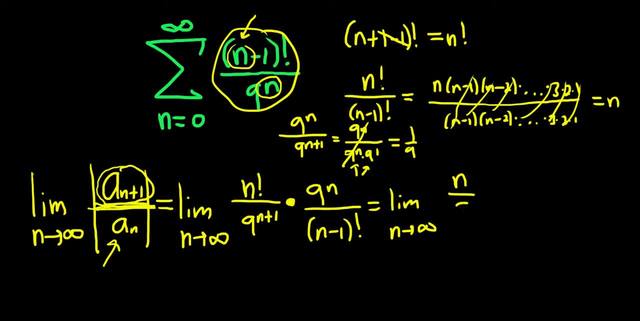 So this is 1 over 9.. So we just have a 9 here, Ridiculous, So it cleans up really, really nice. And this is equal to infinity, which is bigger than 1.. So that means it diverges. 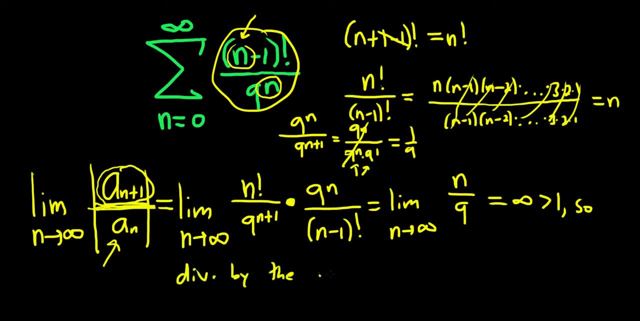 by the ratio test. Recall: the ratio test says: if it's less than 1, you get convergence. If it's bigger than 1, you get divergence. If it's equal to 1, no info. So this is convergence, This is divergence, This is nothing. Nothing at all. Nothing there. So the other way to